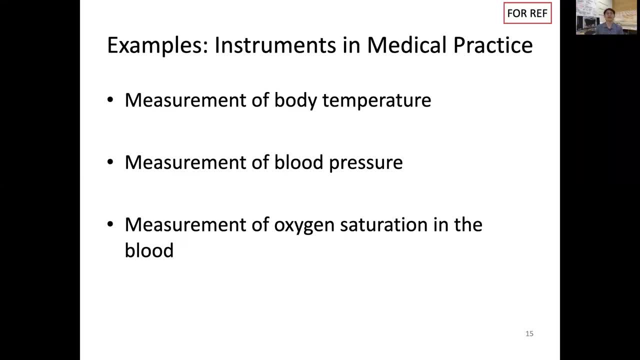 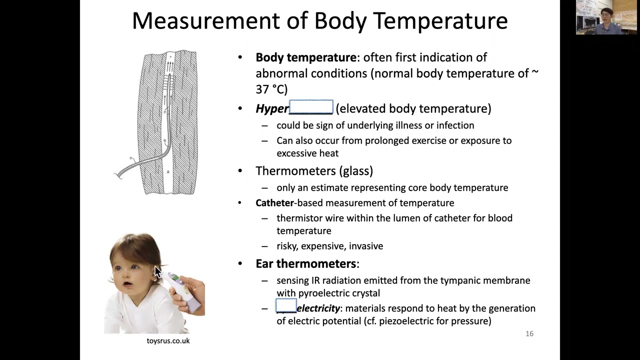 Hi, now let's discuss about instruments in medical practice. I want to give you about like three examples of measurements of body temperature, blood pressure and oxygen saturation in the blood. So measuring body temperature, it's easy, You can see, nowadays a very easy way to measure. 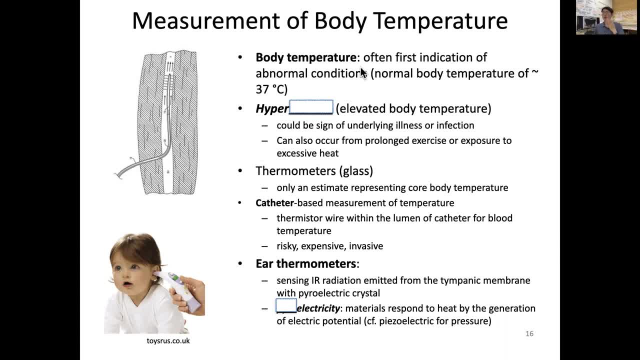 our body temperature. But why body temperature is important? Because it's oftentimes first indication of abnormal conditions. especially, our normal body temperature is about 37 degree And if it's elevated that could be a sign of underlying illness, especially infection. And 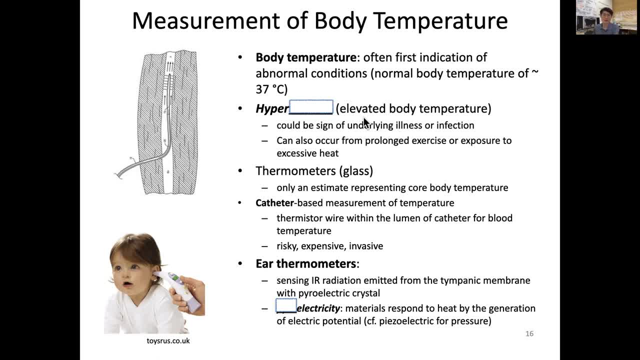 also so that elevated body temperature is called hyperthermia. Okay, so this can occur: prolonged exercise or exposure to excessive heat. So thermometer made of glass you are familiar with this is only an estimate representing core body temperature. So we have thermometer under the 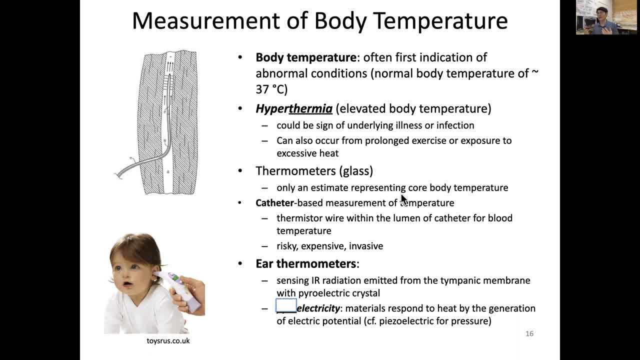 tongue or armpit And that may not be always accurate. So sometimes, in special case, we may need to measure core body temperature directly. Here's an example of a figure that you see: cat or based measurement of temperature. So thermistor wire is within this lumen of catheter for measuring. 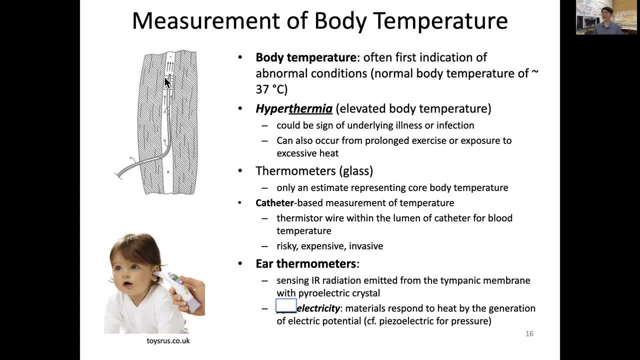 blood temperature And you can see like this can measure blood temperature directly. However, you see, this is risky And this is expensive and also invasive measure, So it's not always happening, But there are times to have this And your thermometer is sensing. 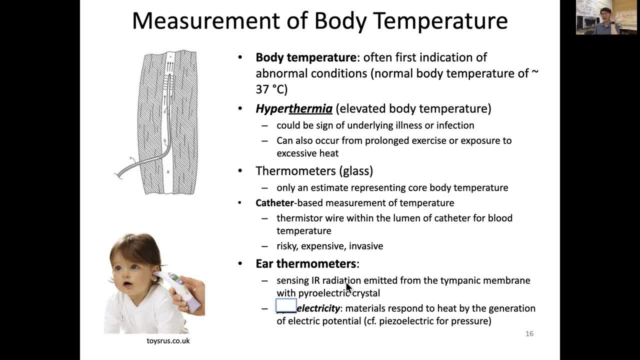 congruent temperature, And this is the same thing. so you need to pay attention to this. So there's a power outage in your patient's another eye and really you need to pay attention to this. And then the second thing is remember what I said. for example, we have an infrared light radiation. 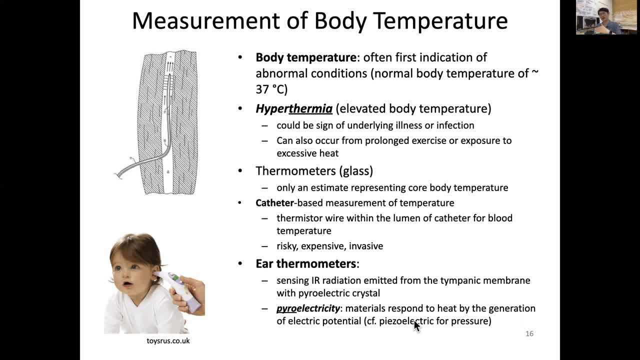 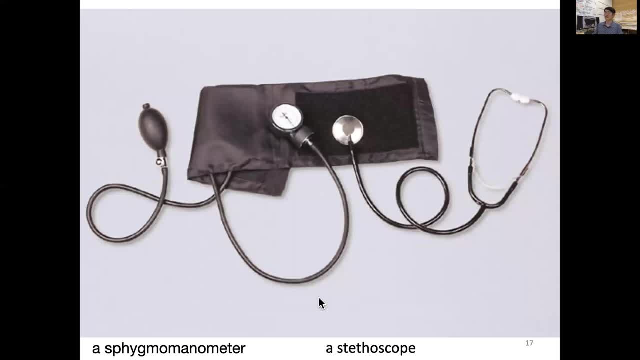 emitted from our tympanic membrane with a pyro electrical crystal. What this pyroelectric means, so induced electricity. Next, I want to discuss about a sphygmometer, which is for measuring blood pressure. Okay, so that's at this part of and this pump, and 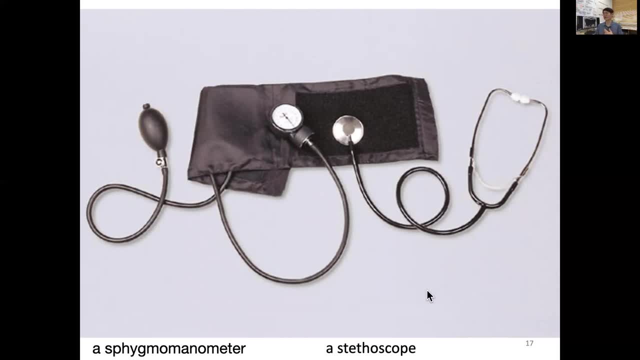 this gauge and there's another one, which is a stethoscope, which is directly measuring the sound by using this diaphragm sensor and your ear. So this combination of sphygmometer and a stethoscope is a traditional way of measuring our blood pressure, So usually using your arms and measuring the rate. 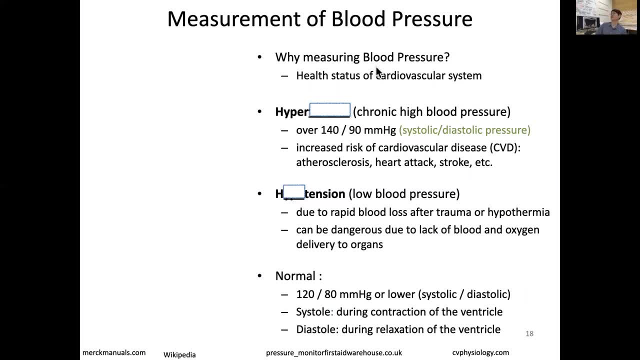 artery. So why measure blood pressure? This is also very important for knowing health status of your cardiovascular system. So this diagram shows that the artery in our arm- and you see these are arteries, so there's like pulsation from directly from our heart and that pressure cuff measuring giving this. 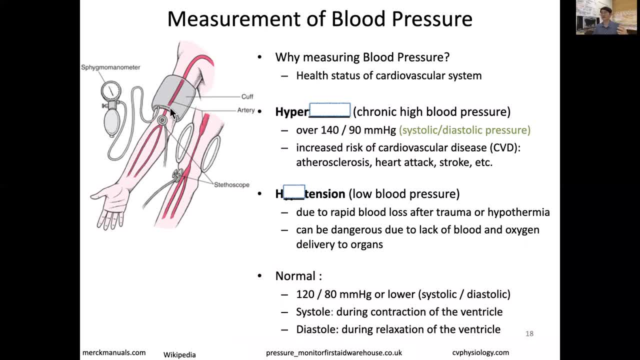 pressure and you first elevate the pressure high enough that you squeeze these necessary fluid building up to the heart and to the sphygmometer and by that artery, until it doesn't flow anymore, and then you release slowly, then what happens is, as you remember, that this narrowing makes the flow faster and that 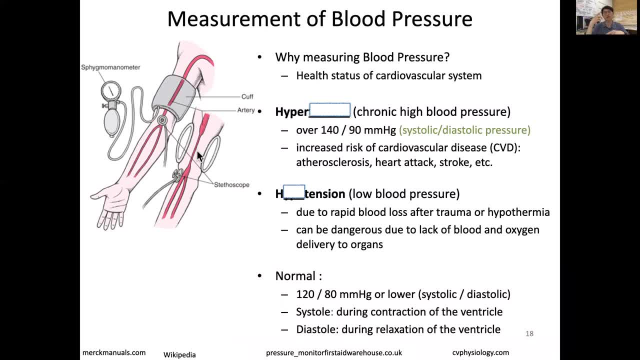 gives a high Reynolds number, or make the flow turbulent. turbulent is irregular and making an eddy and that gives you a specific sound of depending on your purse together so with that sound we can measure the sound with a speaker denominator. so when we measure our blood pressure and we will find out chronic. 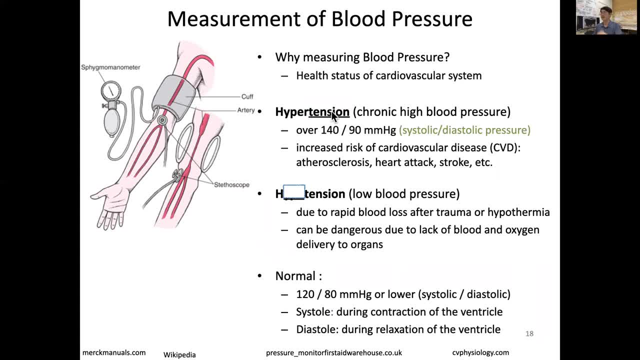 high blood pressure, which we call hyper, yes, tension, and that's defined by systolic and diastolic pressure as high, higher than 140 and 90 millimeter HG, and what this indicates is a risk of cardiovascular disease, such as a atherosclerosis in your vessels and heart attack or stroke. 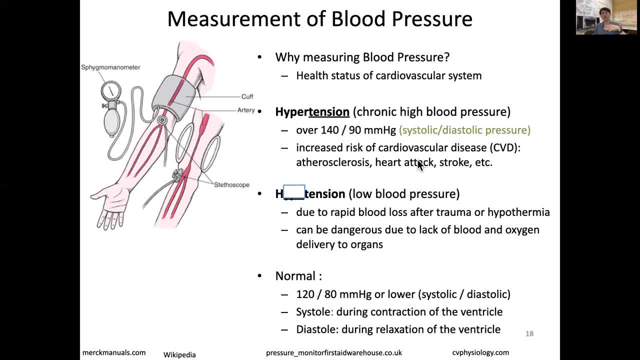 has higher risk. on the other hand, you could have very low blood pressure, which we call not hyper, but, yes, high poor tension. and when does hypotension can occur? and if there is a big trauma that you lose your blood volume and rapid blood loss can give you a high poor tension and also. 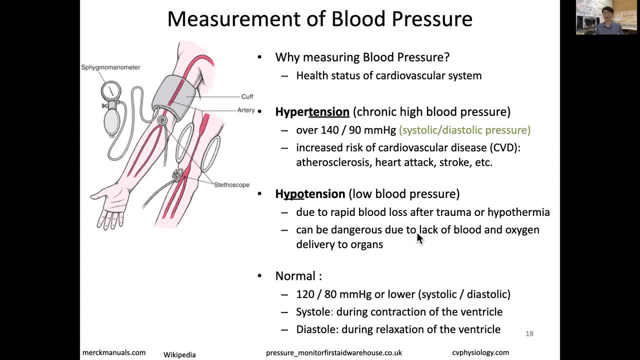 hypothermia, which could be dangerous because if you lack of blood, you your lack of oxygen delivery to organs and you lead to shock. so this is very important to catch if or one patient have hypertension. so what are the normal range for blood pressure, which is about systolic pressure as as lower than 120. 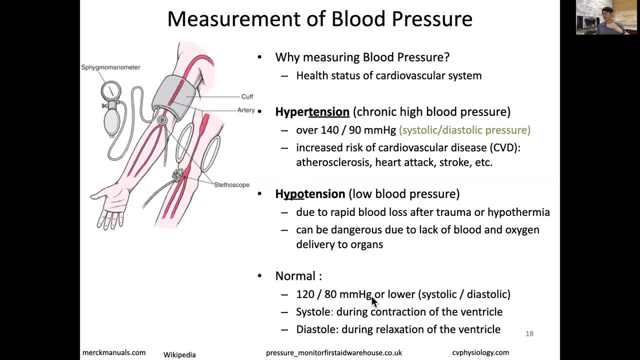 and diastolic pressure as Lord and 80 hg. and nowadays these traditional measurement can be replaced by more advancement of technology, which is using, remember, mechanical sensor, using the measuring the pressure by the stretch of the surface of this cuff. so that is this, electronic ways and there's a mechanical strain. 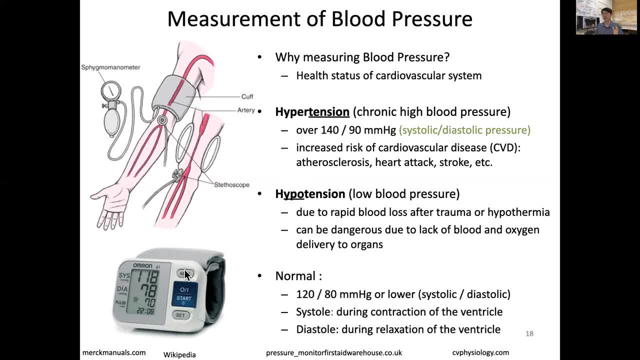 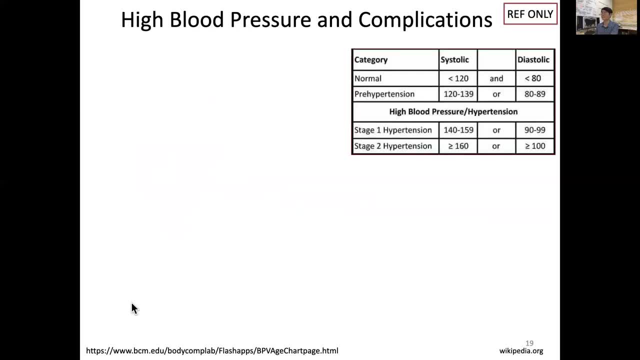 gauge inside which measures the pressure directly, and even you analyze this data well enough. you can even measure the pulse rate as well. so, given the high blood pressure, i just want to uh mention a little bit of the definition of high blood pressure. and you can see normal below 120 and 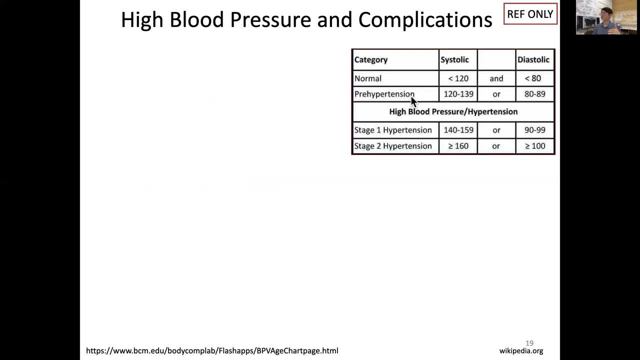 below 84 diastolic. there's a pre-hypertension in this range and high blood pressure or hypertension is defined as higher than 140 and higher than 90. that's stage one hypertension. if you are stage two, that's dangerous. that's higher than 160 and 100 for systolic and diastolic pressure. 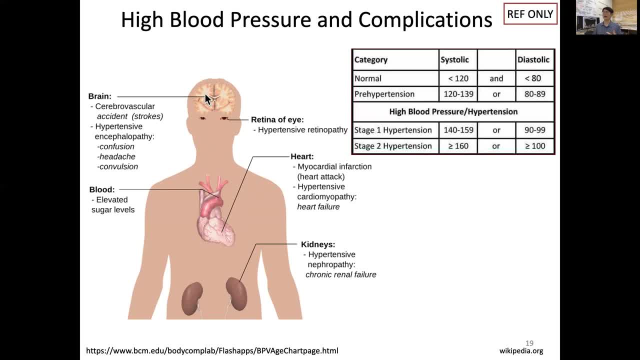 and why this become a problem. because you see there are many of uh risk with higher involved. with high blood pressure, such as cerebrovascular accident, stroke can happen more, and hypertensive encephalopathy and apathy means that this kind of pathology involved. so you can. 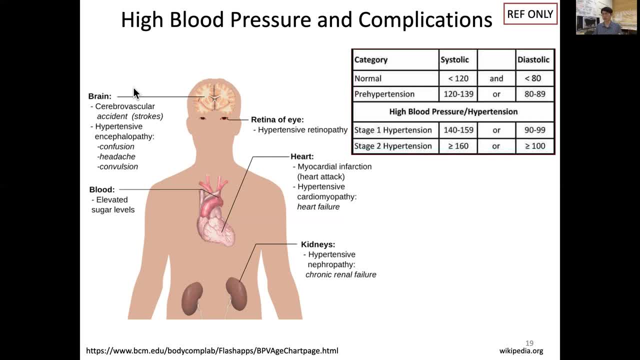 have confusion, headache and convert conversion and retina of the eye is also sensitive for the pressure and if there is hypertension then hypertensive retinopathy which affects our retina and uh blood it. this can leaves a elevated sugar levels and heart eye or myocardial infarction, which is simply heart attack, can happen. and hypertension makes 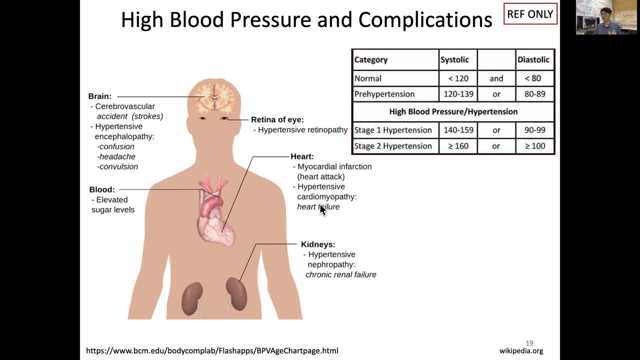 your heart abnormal uh heart muscle or cardiomyopathy, or it can lead to heart failure- and also your kidneys as well. kidneys filter a lot of your blood a day like almost uh like over 1800 liters, and that kidney can can suffer from hypertensive nephro nephropathy that leads to chronic renal failure. 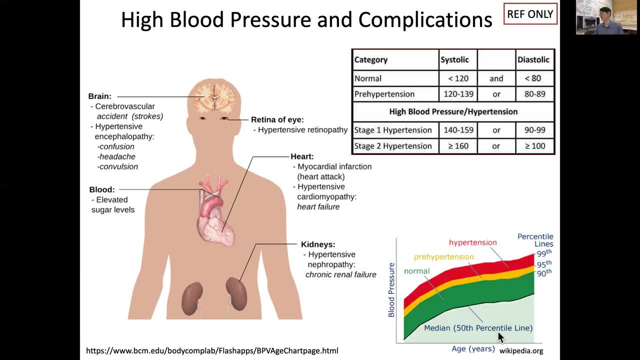 so one one noticeable thing is: you see, uh, over age, there are data showing blood pressure of of this keep increasing. so even if you you have a lower blood pressure, you're okay, but you see, over age, your blood pressure is always tend to go higher and higher. okay, so that's why. 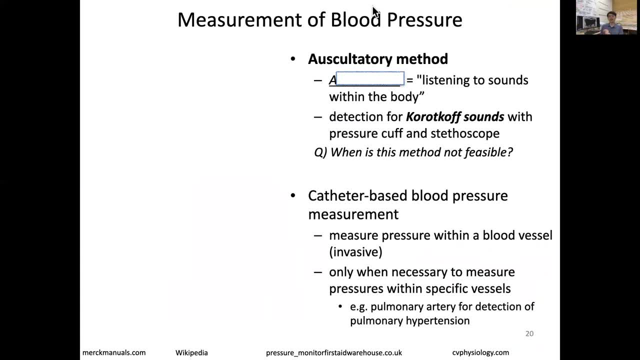 you need to pay attention to this, and so, because of that, let's talk about measurement of blood pressure, and traditionally this is called oscar oscultatory method, and auscultation, uh is is meaning as a listening to sound within the body, so this is to remember- with a pressure cuff. 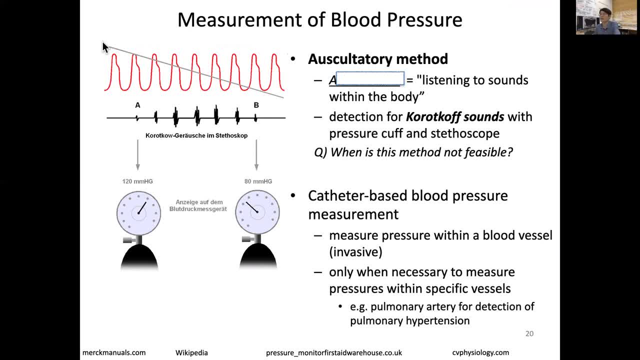 and you release the pressure. uh, that is shown as a gray over time. so you release and this red is your arterial blood pressure. so when cuff pressure is higher, then it squeezes. so it squeezes completely the other, so you don't listen any sound. but once it's in between, then 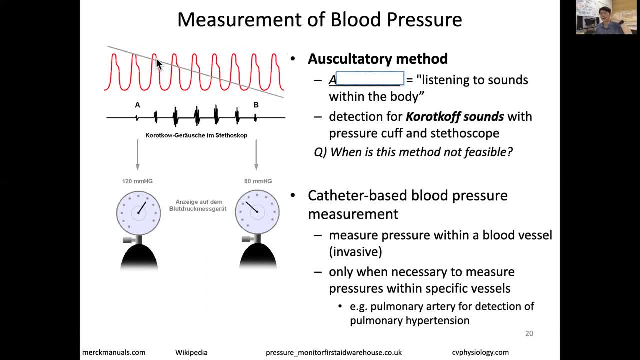 the flow starts to move and that purse, generating turbulence, will causes a sound which we call auscultation, listening to sound. and so you see, listen the sound, and that's called karate cuff. and until the cuff pressure is lower than the actual arterial pressure, then you don't hear a. 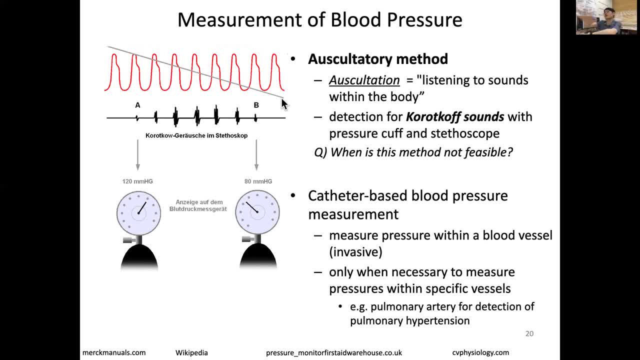 sound because you're not squeezing the artery anymore. the artery will smoothly flow. until you have this squeezement, then there is a sound here. so by detecting this karate cough sound with higher beginning and then later you can read a systolic pressure and diastolic pressure. so 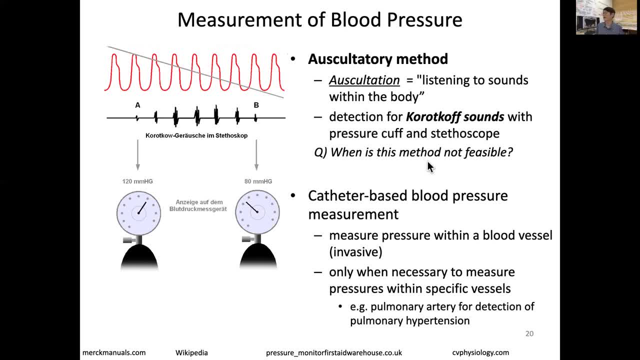 you can see that this method is not feasible. um, so that's actually when a patient has a underlying lung problem and you need to check co2 and oxygen of blood frequently, then this method may not be, uh, useful. on the other hand, there are like a more common methods that can be used to check. 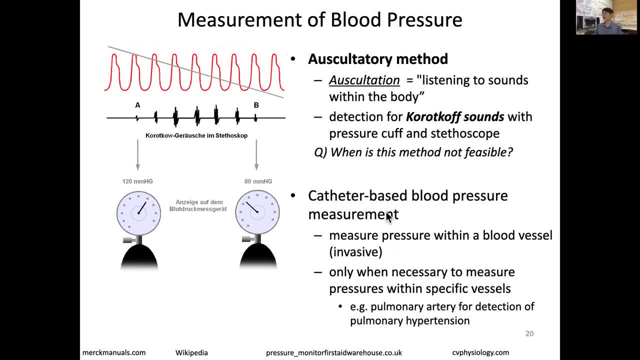 the blood pressure and the oxygen level of blood. so this method can be used to check the blood pressure and the oxygen level of blood. and then the second method is called the catheter-based blood pressure measurement, so this method is called catheter-based blood pressure measurement. 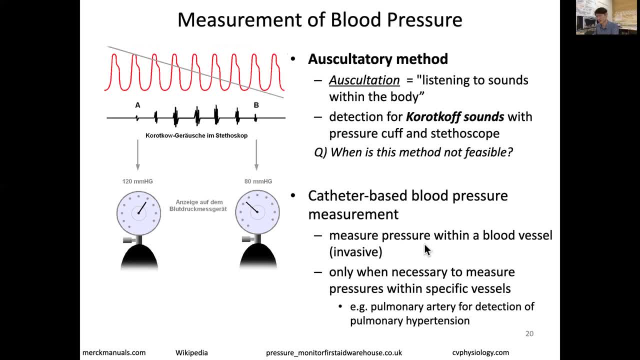 and it's a more precious, a precise measurement called catheter-based blood pressure measurement that you want to measure blood pressure within a blood vessel. so this is invasive. only use when within specific vessel measurement is necessary. for example, if summons are used to measure blood pressure, then the blood pressure can be measured through the heart. 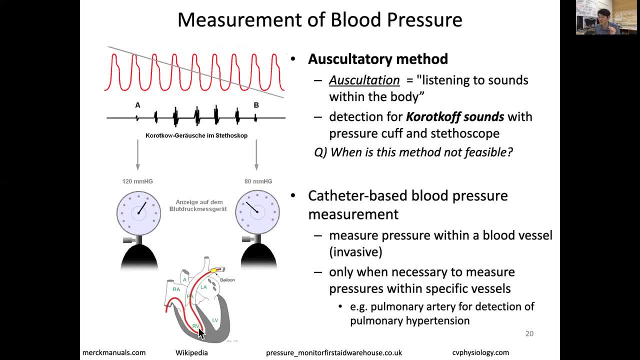 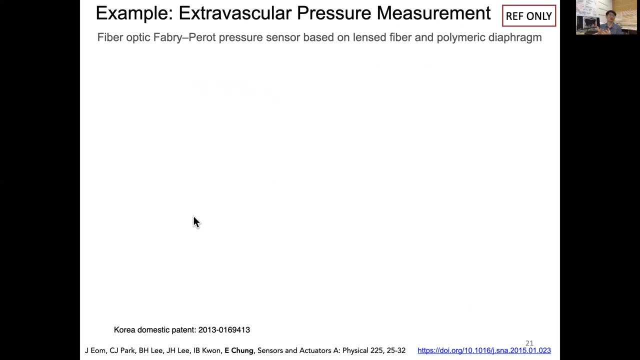 and the pulmonary artery need to be measured for blood pressure. so, through the heart, the catheter based blood pressure can get in to into right ventricle, right atrium. it goes to pulmonary artery so that it can measure the pressure of pulmonary artery. so, uh, so that extra vascular pressure measurement. i want to give you an example, which happened to be: 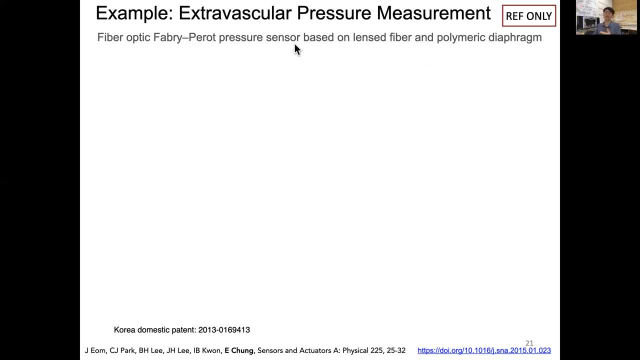 this fiber optic based fabric parallel pressure sensor based on lens, the fiber and polymeric diaphragm. so what that means is that we created a optical fiber where the light goes in and there's a lens of the fiber was made and that fiber is into uh reflected from a polymeric diaphragm. 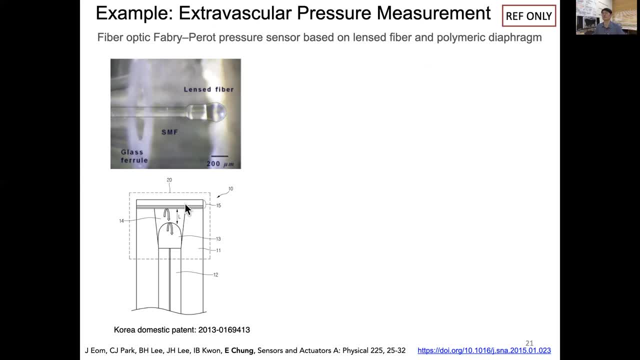 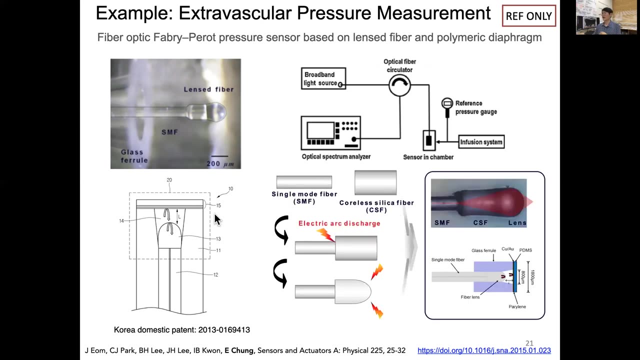 which is diet polymer, so that it responds to pressure, that tiny, tiny displacement can be measured by optical interference and which can be detected by this optical spectrum analyzer with a broadband light source. so, and to create this, and we need to have a um, create this lens, the fiber, and having, uh, this electric arc discharge to make it like lens, so that we create 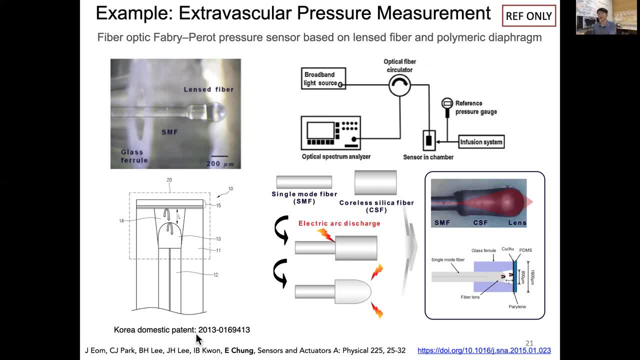 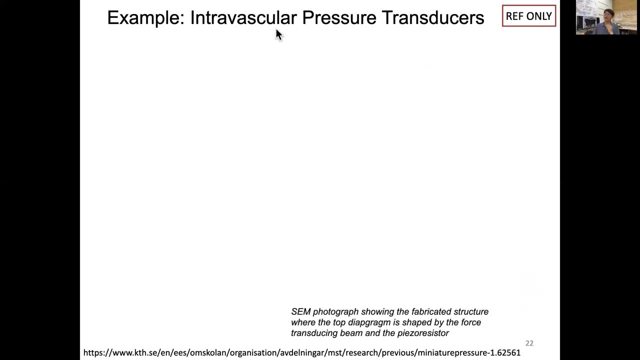 this and uh, and we actually publish this one and generate patterns. so that's kind of an example of very fine extra, extra vascular pressure measurement system you could potentially use it for inside the body. and another is the intravascular pressure transducers, um, which is a. 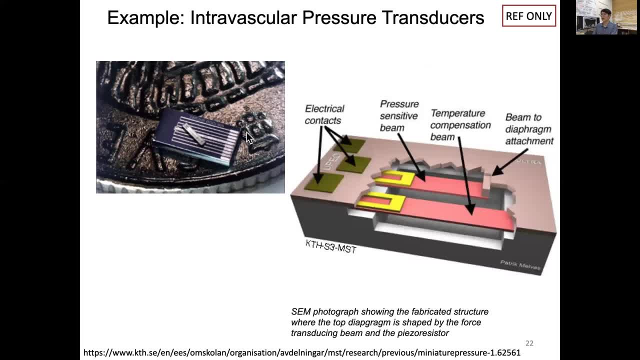 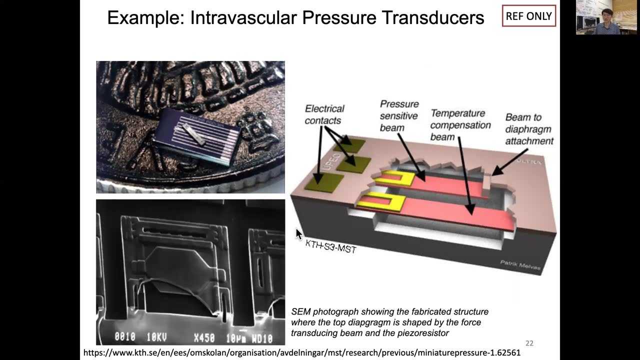 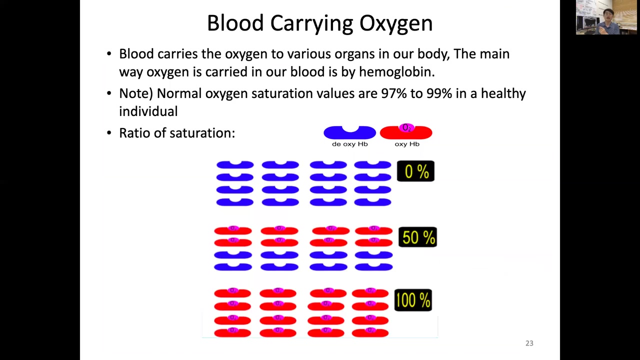 very, very tiny. you see this out of this coin and tiny, tiny sensors can be directly put it inside the vessel and measure pressure. so this is the diagram showing pressure sensitive beam and compensation and the actual electron microscope shows: uh, these fabricated device. so now the next i want to discuss about the oxygen concentration, so blood carrying the oxygen to. 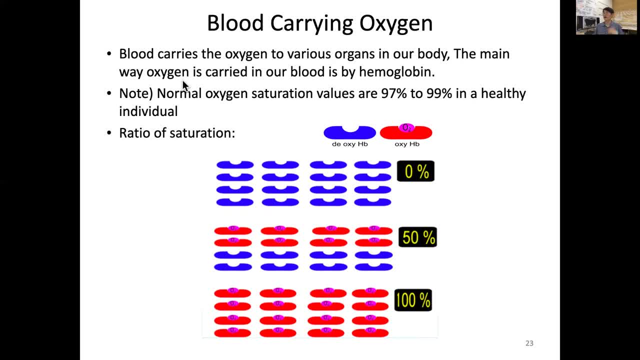 various organs in our body. the main way of oxygen carriage is by hemoglobin. you remember at the first time at the molecular principles. hemoglobin is a uh kind of tertiary structure with four subunits. each can hold one oxygen uh molecule. so normal oxygen saturations uh for human is about 97 to 99 percent in healthy individual. and what does this? 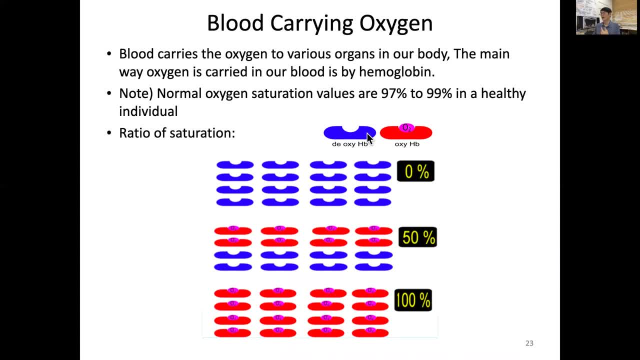 oxygen saturation means- and here's a simple diagram of hemoglobin- can have, do not have normally oxygen that we call deoxyhemoglobin. once it gets oxygen molecule, that's oxyhemoglobin. so if none, zero percent, half of this hemoglobin uh was saturated and that's 50 and all the hemoglobin. 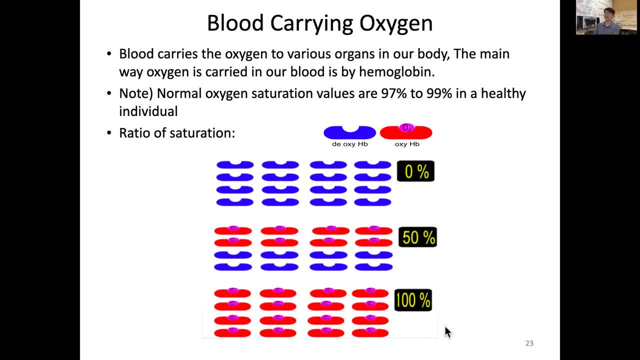 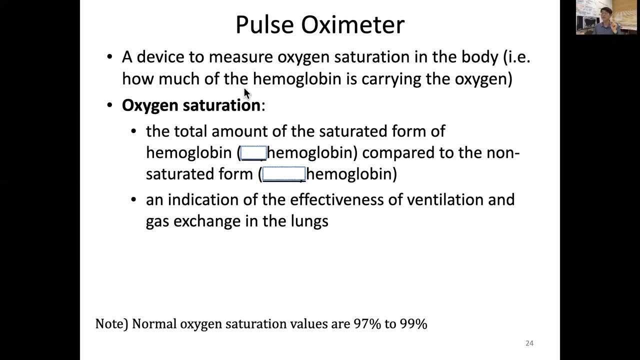 will hold oxygen 100, is that simple? so a device to measure this oxygen saturation in our body, or how much of the hemoglobin is carrying the oxygen, is called pulse oximeter, so oxygen meter measurement. so oxygen saturation is the total amount of saturated form of hemoglobin, or we call, yes, oxyhemoglobin, compared to non-saturated form. 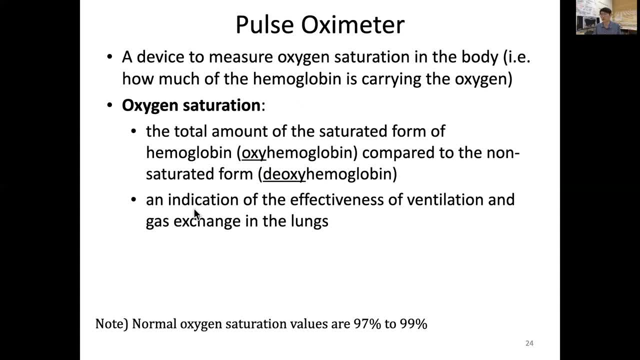 or deoxyhemoglobin, and this oxygen saturation is an indicator of effectiveness of a person's ventilation and gas exchange in the lungs. so let me give you a formula. so that's, a percentage of a saturation of oxygen is- uh, you know, oxygen saturation is the total amount of saturated form of hemoglobin, or, you know, oxyhemoglobin divided. 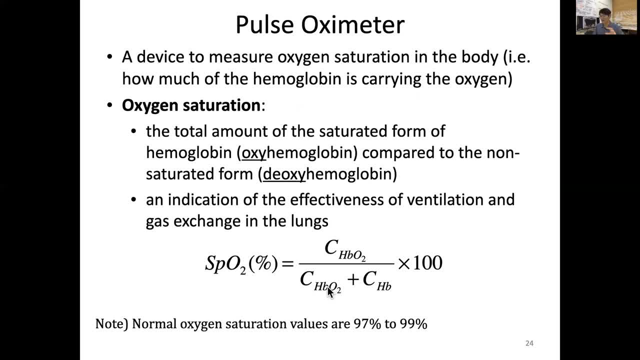 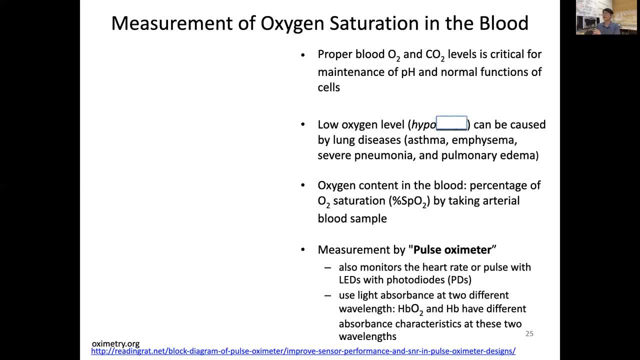 by total hemoglobin c concentration. and total hemoglobin is composed of oxy and deoxyhemoglobin and multiplied by 100 for making a percent. so to measure this oxygen saturation in the blood, the proper blood oxygen, co2, which is crucial for maintaining our ph and normal function of our cell. 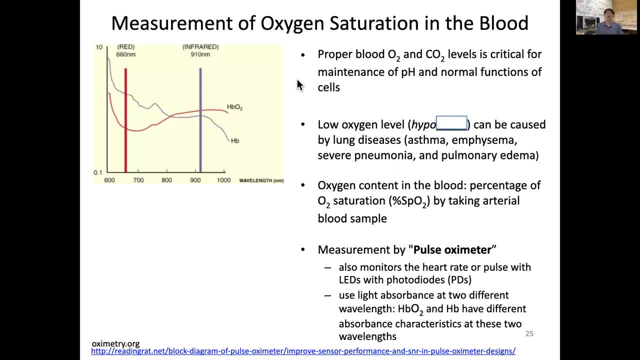 and we're going to use this in the next slide cells. so to measure, we use a trick based on biophotonics and the optical property of the blood. you remember that some blood, when you cut, you can see a dark, darker color of blood. but if you happen, 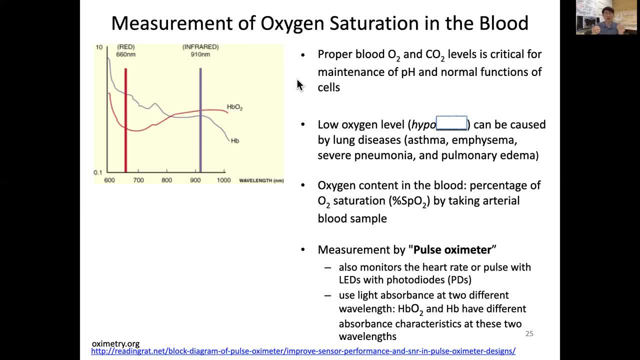 to have a, let's say, a real arterial blood coming. that's a bright red. so the different color means something and that using that difference in color or the color means the absorption of the light in visible ranges are different and using that we could actually, uh, quantify a the status of oxygen saturation. so that's showing up in this. 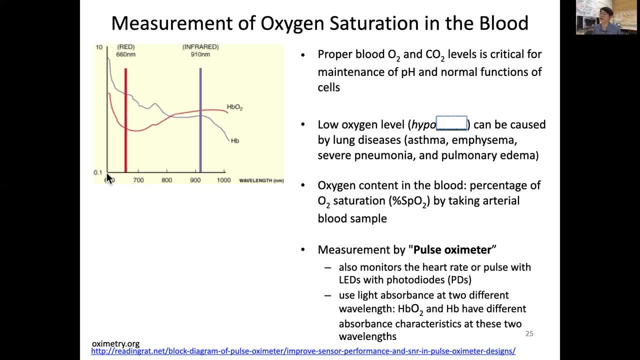 absorption spectrum. what it means is you see this x-axis as a wavelength or color of the light and y-axis is the absorption. so you can see blood, so you can see that this is a very high absorption and you can see that the red blood cells are. 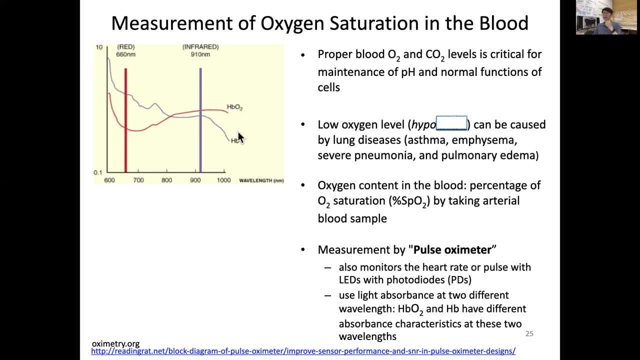 usually red because of this high absorption in the green and blue range and interestingly, the oxy deoxyhemoglobin has quite different absorption and you can see oxymogon has much lower in this 600 to 700, which is red color, absorption is low. what that means is the red color when hit this uh. 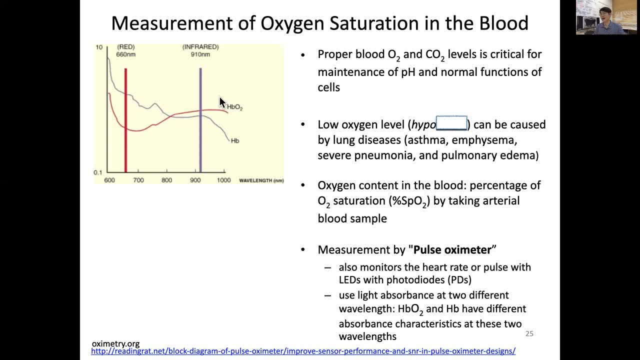 our eye it looks bright red color. so that's oxyhemoglobin spectrum and deoxy. so in principle there's only two unknowns: concentration. so you could just use two colors of uh, of light sending through the tissue, and detect and you can recover the concentration of two variable. so that's the 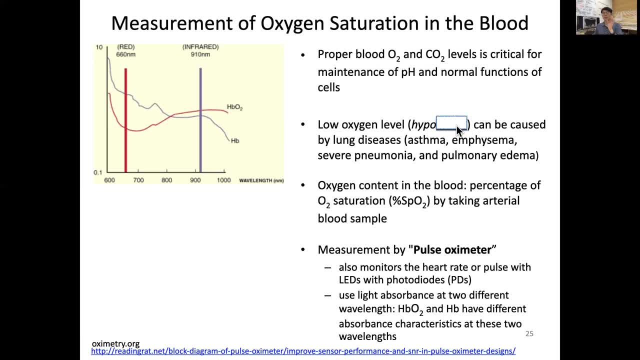 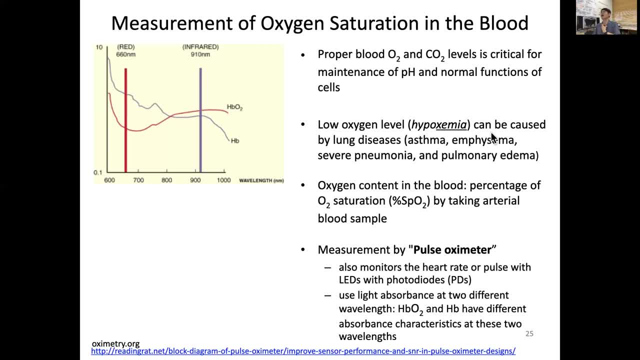 and pulmonary edema. all of these affect airway and lung parenchyma which will affect our proper oxygen. gas exchange and oxygen content in the blood is described as percentage of oxygen saturation by taking arterial blood sample. so that's a gold standard. and the pulse oximeter i brought a nice. 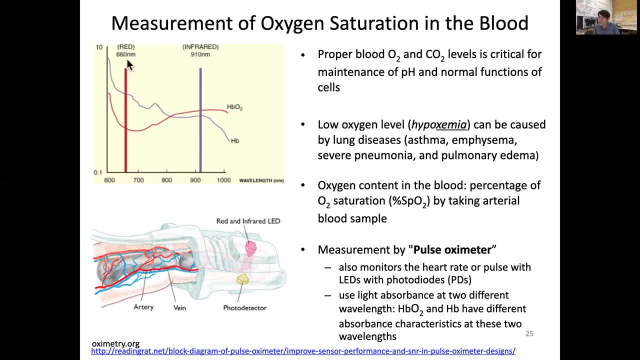 diagram here and how. how do we measure sending this two color of light, such as, let's say, 660 red led light emitting diode, or infrared, 910 nanometer, and then you need a detector, which i just described as a photodiode. so you see here, red and infrared, two kinds of 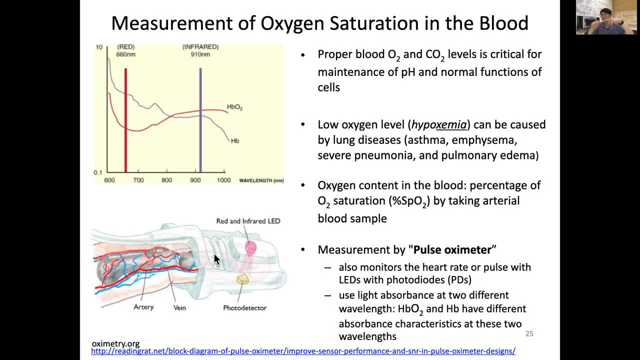 leds are sending the light through the finger, and inside the finger there is a blood vessel and so it will absorb. and you have a photo detector so that measurement of by pulse, oximeter monitors. uh, not only this concentration, your signal will fluctuate because of the heartbeat, so you can even 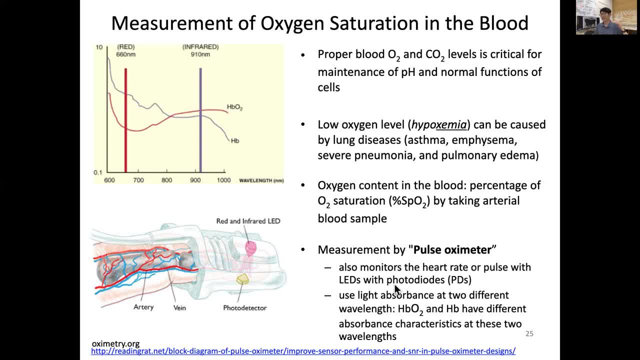 measure heart rate or pulse rate with leds and photodiodes, and we use. light absorbs germans at two different wavelengths. oxyhemoglobin and deoxyhemoglobin has different absorbance characteristics at these two wavelengths. so that's the trick and we are using it. and now this is very. 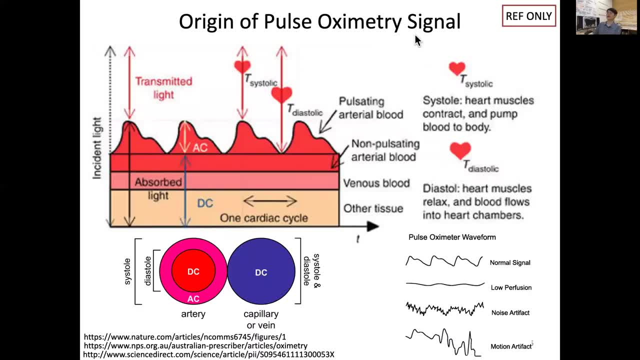 cheap. so the origin of pulse oximetry signal is described here and i will skip this. but i'll just give you an idea that the actual signal from photodiode what you get is normal signal. you see, this heartbeat is showing and also the degree of this height will gives you the oxygen saturation. 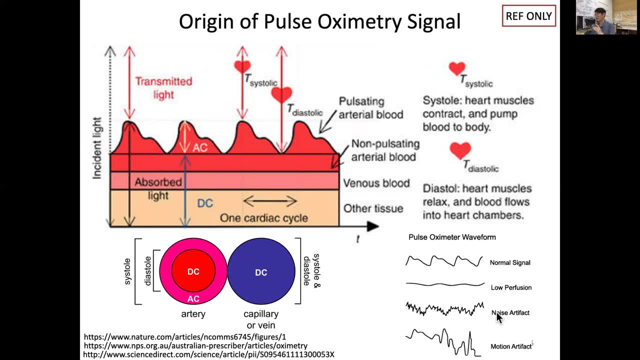 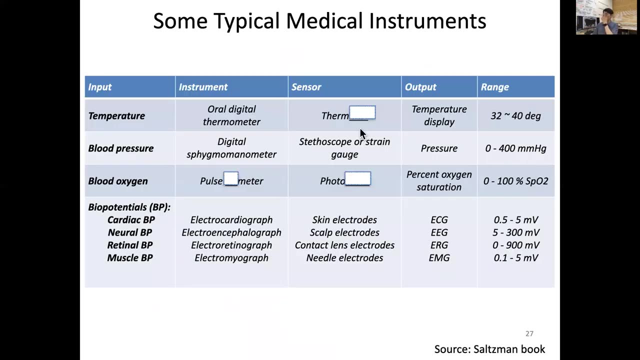 but it also shows low perfusion- noisy artifact and motion artifact. so it gives us an engineering challenge and problem to how to analyze this signal and turn it into a oxygen saturation percent. so now i want to summarize typical medical instruments and example temperature. i show oral digital thermometer which uses a thermistor as a sensor and that output will give. 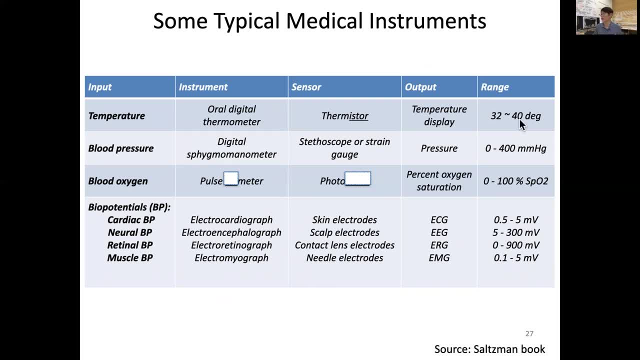 a temperature within the range of 32 to 40 degree. blood pressure, as a simple one now has a digital speaker monometer and the sensors are stethoscope or strain gauge and the output pressure is zero to 400 millimeter hg and blood oxygen. we use pulse oximeter and that sensor was a photodiode and 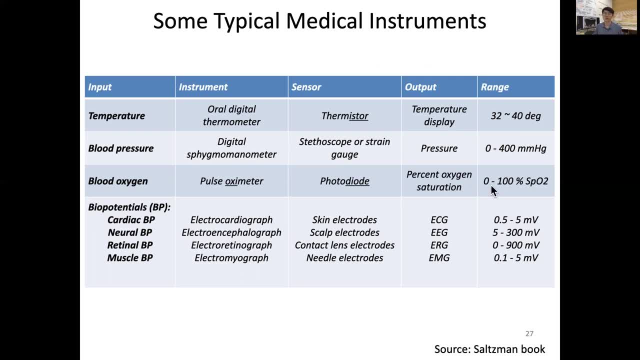 that gives a percent oxygen saturation from zero to a hundred percent, and electrical sensors, which i haven't discussed much, but that's called biopotential, and there's cardiac biopotential, neural, retinal and muscle, and that's we call electrocardiography, electroencephalography or 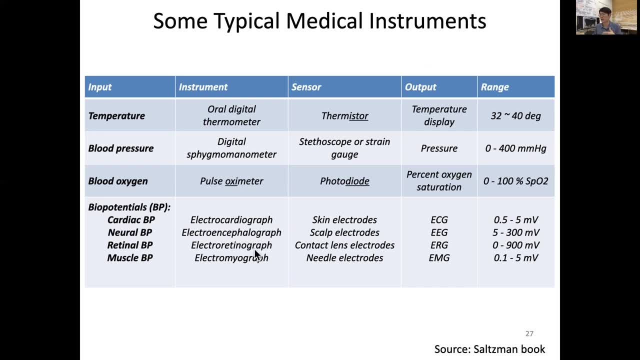 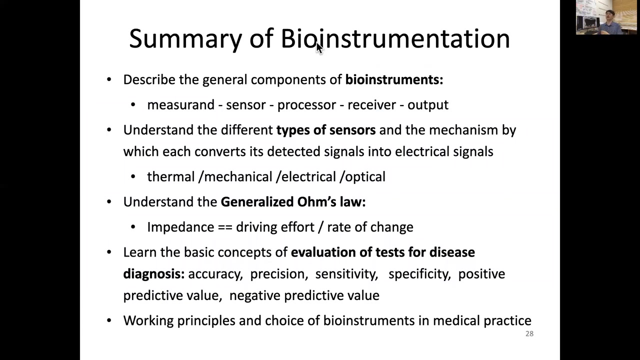 eeg and electro retinography and electromyography and you can see there are different kind of skin, scap, contact lens and needle electrodes and that's measuring the range of a millimeter to several hundred millivolts which is happening as a biopotential inside our body. so in summary,